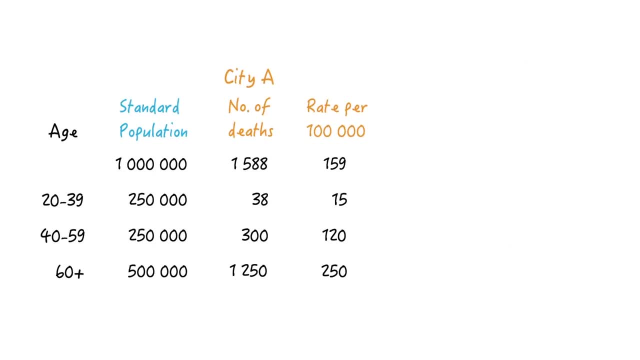 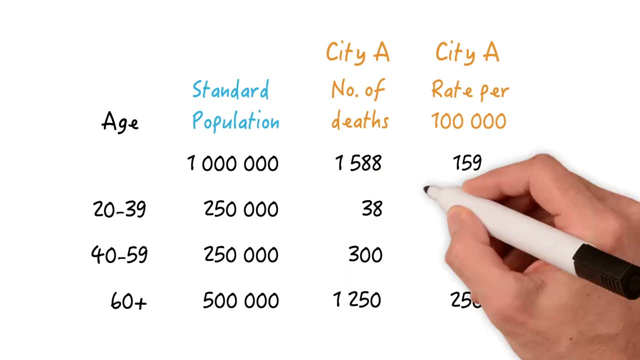 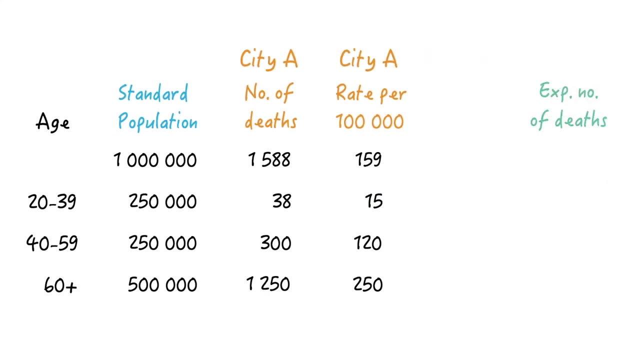 We could either create a fictitious one or just use one of the two cities. Let's choose city A as our standard population. This is the age distribution, These are the numbers of deaths and this was our death rate in city A. Now, how many deaths would we expect if the age distribution was the same in city B as in city A? 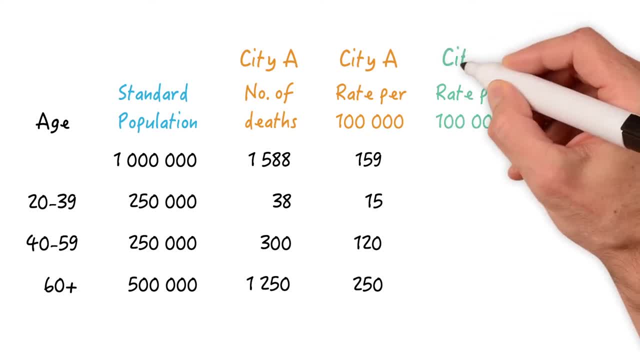 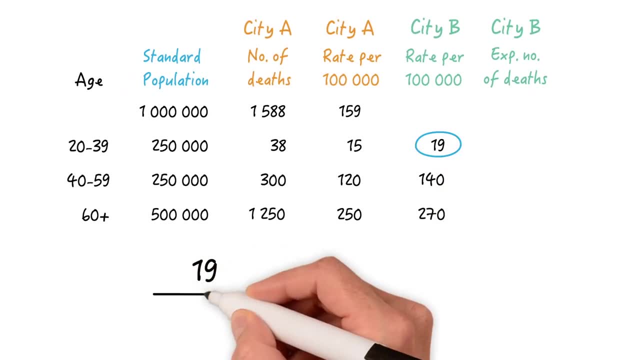 To answer this question we need the age-specific death rates of city B and apply them to the age strata of our standard population. So 19 per 100,000 multiplied by 250,000 equals 48, expected deaths: 148.. 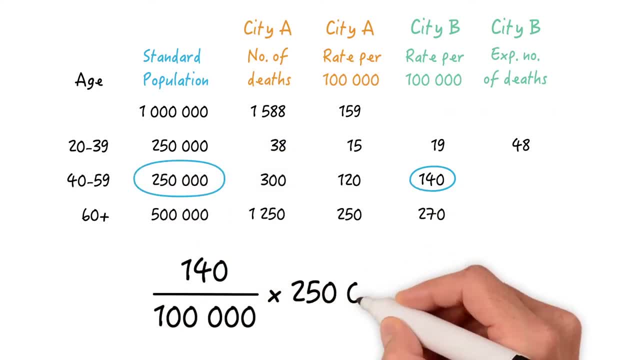 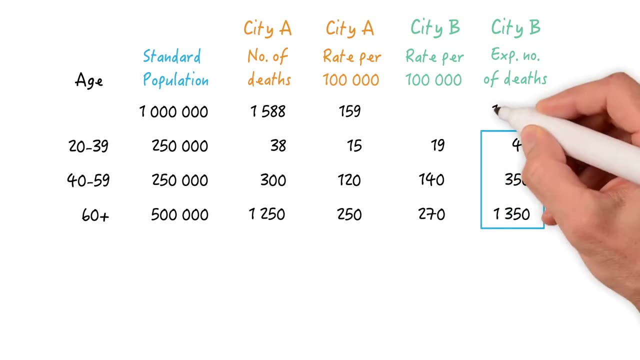 30 per 100,000 multiplied by 250,000 equals 350 expected deaths, And 270 per 100,000 multiplied by 500,000 equals 1,350 expected deaths. So overall we'd expect 1,748 deaths if city B had the same age distribution as city A. 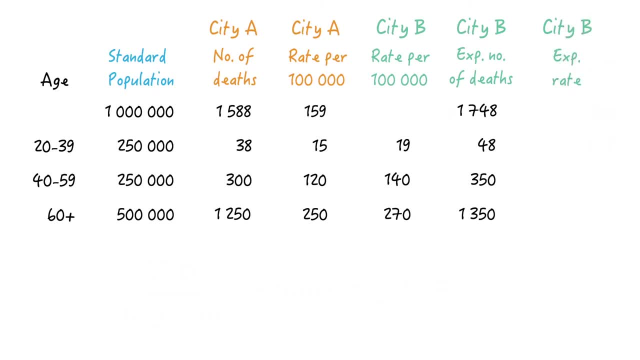 And what would be the overall death rate per 100,000 population? That's 1,748 divided by 1,000,000 times 100,000.. So 175.. This means that the age-adjusted death rate using city A as the standard population. 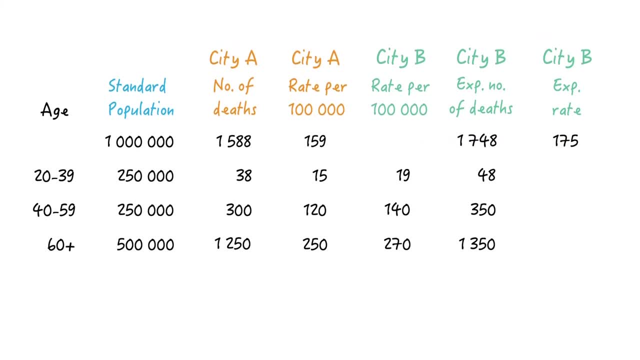 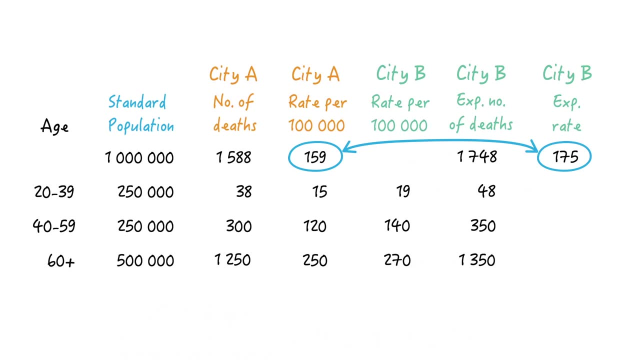 would be 175 per 100,000.. Now we can compare that to the crude death rate of city A of 159.. And what we see is that, after accounting for age, the death rate of city B is actually higher than in city A. 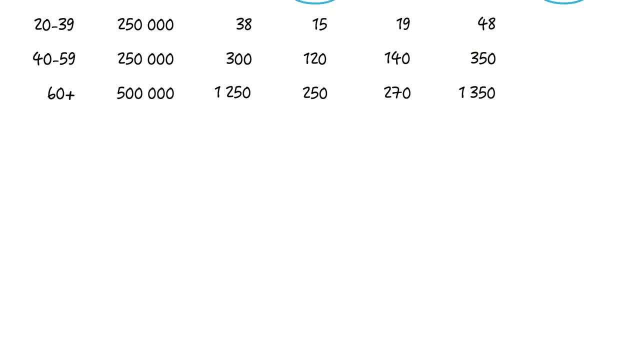 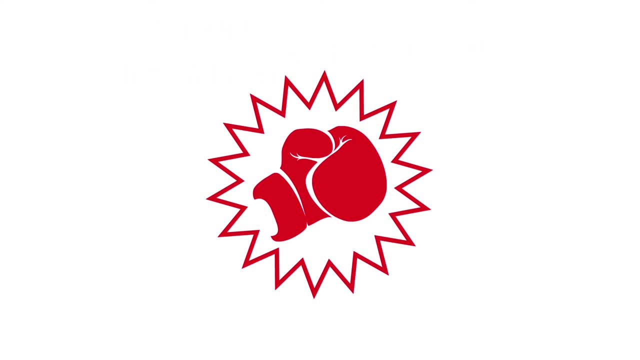 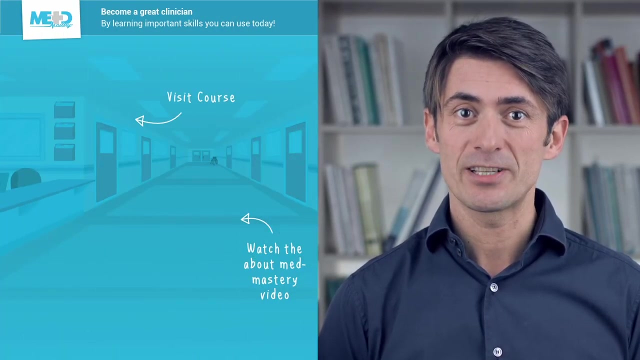 So the same findings as with the stratified rates. So adjustment is another powerful tool to combat confounding. So I hope you liked this video Absolutely. make sure to check out the course this video was taken from and to register for a free trial account, which will give you access to selected chapters of the 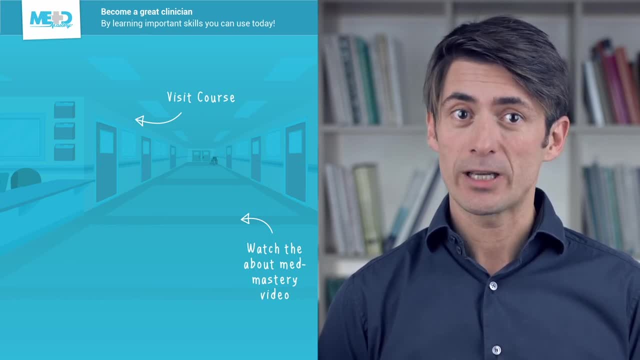 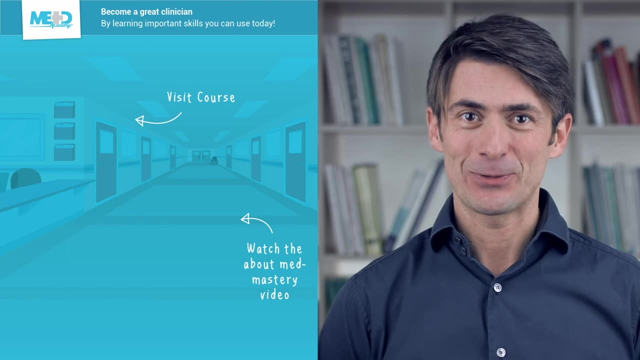 course, If you want to learn how Medmastery can help you become a great clinician, make sure to watch the About Medmastery video. So thanks for watching and I hope to see you again soon.